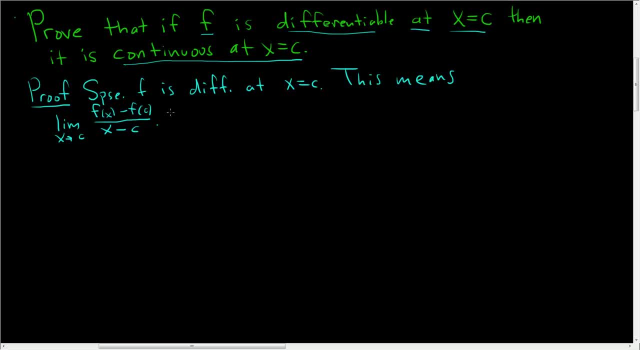 Now, in order to give you some direction as to how to prove this, I'm going to write down what we need to show. So we need to show that the limit as x approaches c of f of x is equal to f of c. 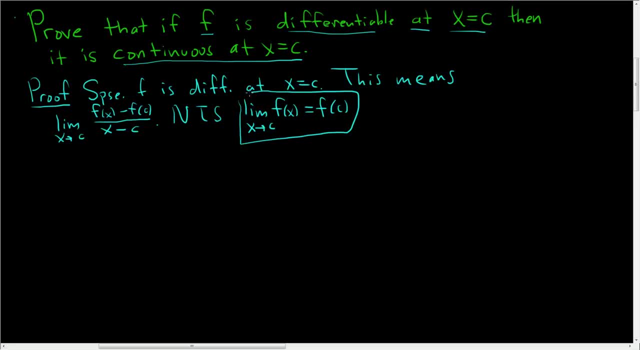 So if you look at this statement here that we have to prove and you look at what we have over here, you'll notice that here we have f of x minus f of c. So it might be easier to show the following: 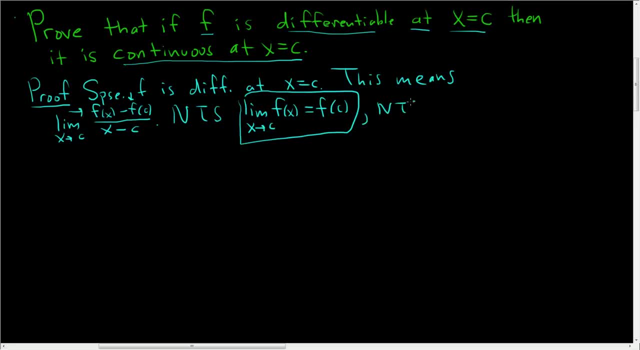 So we need to show this. So we need to show- Let's rewrite this in a way that matches what we have over here- So we need to show- that the limit as x approaches c of f, of x minus f of c is equal to zero. 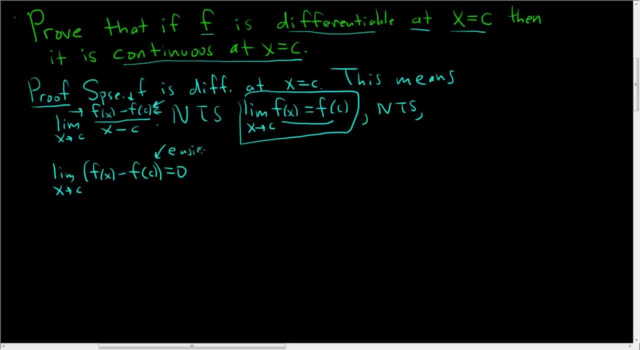 So this might be an easier route, based off what we have up here with differentiability. So let's prove this. So then, the limit as x approaches c of f of x minus f of c, this is equal to the limit. 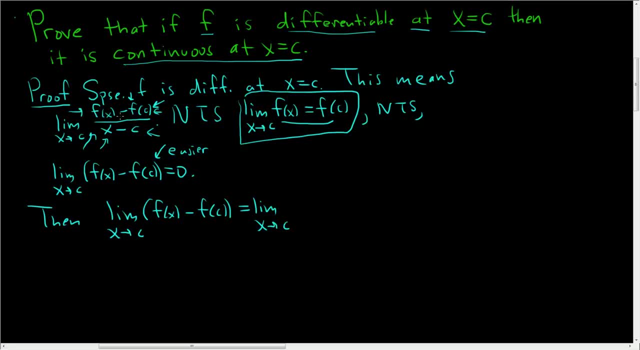 as x approaches c. Now here's the trick: We're going to incorporate this. So we already have f of x minus f of c. We already have that here, So we can't get rid of it. So we still have f of x minus f of c. 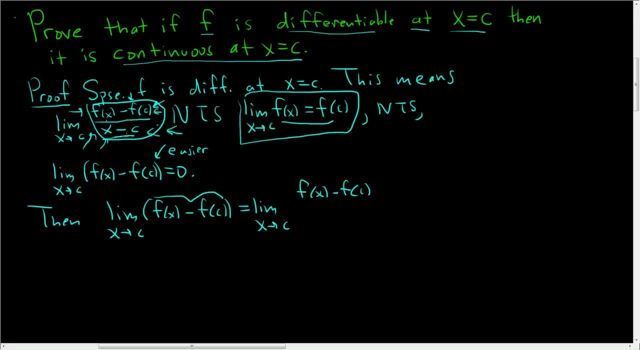 And since we want to incorporate this, we're going to write down x minus c And then we'll just get rid of it. So now we know that we the limit, as x approaches c, of x minus c is equal to zero. 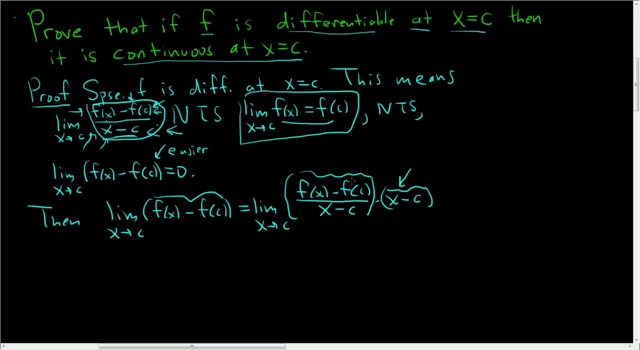 The limit of this exists because the function is differentiable. So this will be f prime of c times zero, which is zero. So we've shown that this limit is equal to zero. To finish, we'll take the limit as x approaches c of f of x. 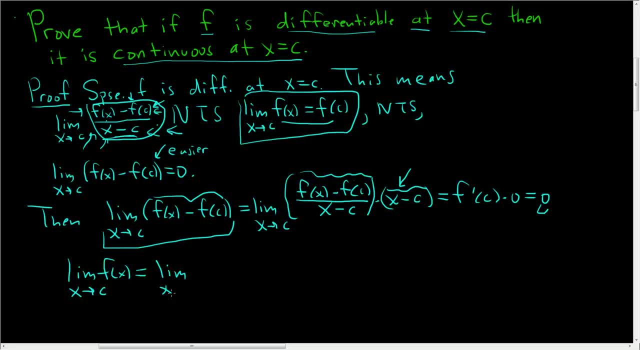 And this is equal to the limit as x approaches c. Now we need to incorporate this, So we'll write down f of x minus f of c, And then we'll add f of c. Adding zero is a really common technique in calculus proofs.